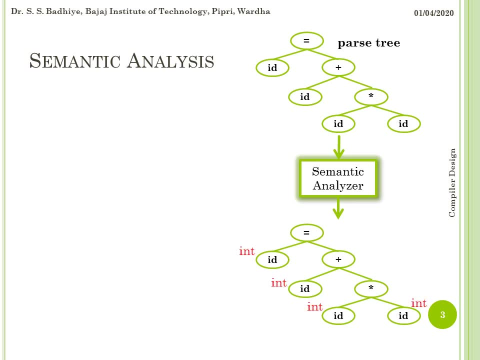 So the output of semantic analyzer is a parse tree with certain additional properties attached to each node of the parse tree, Like as shown in the figure, that int is the properties which is attached to different ID nodes. These additional properties of each node are called as the attributes of these nodes. 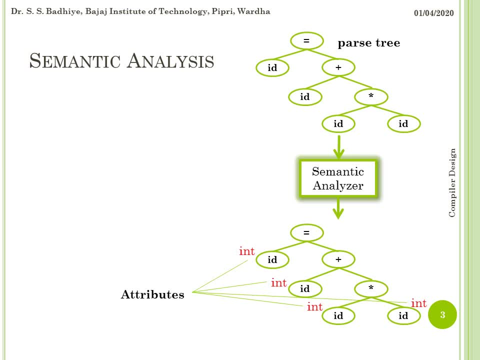 So the output of the semantic analyzer is a parse tree with certain additional properties, known as attributes, attached to it. further, the output of the semantic analyzer is another parse tree, called as an audit parse tree, Which is the output of semantic analyzer. The task of semantic analyzer is to check whether the input is semantically correct or not. 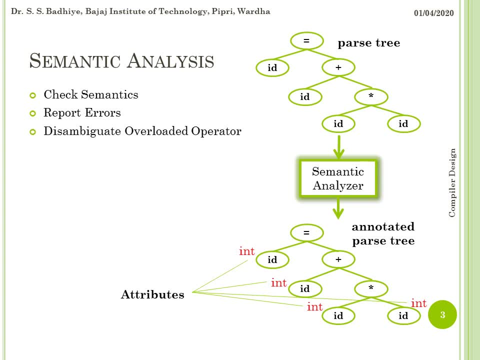 To report if there are certain errors in the program, To disambiguate the overloaded operators and sometimes perform forceful type conversion if required, based on the input type checking, control flow checking, uniqueness checking and name checking. Here we are going to discuss what is beyond. 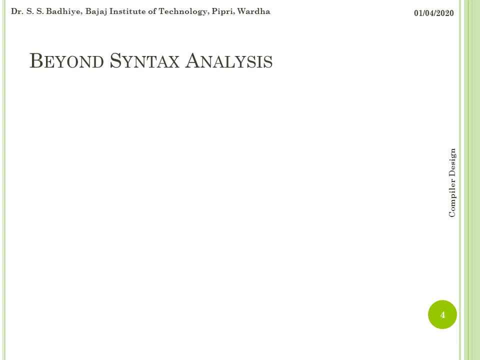 the scope of syntax analysis? or why do we need semantic analyzer, As we know that syntax analyzer is not able to detect all kind of program errors. A deeper level of correctness is present in the program than that of syntax analysis That is, a syntax analyzer accepts. 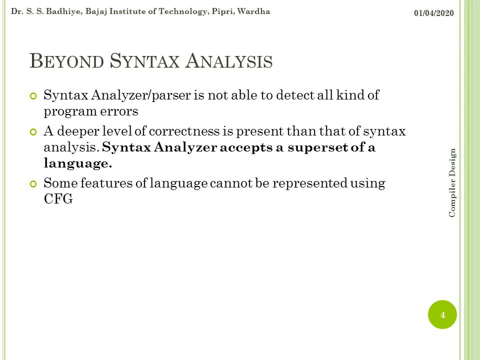 a superset of language. Some features of the language cannot be represented by using context free grammar. For example, if we are declaring an identifier, the context free grammar is not able to check whether the identifier is declared before it is used in the program. Moreover, 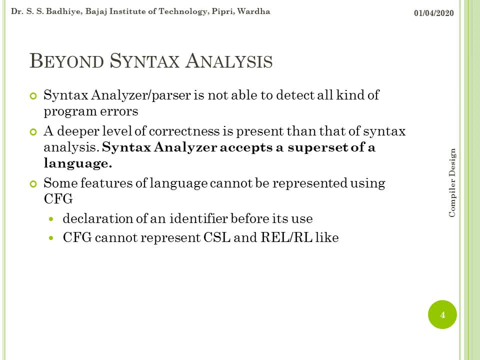 a context free grammar cannot represent context sensitive language. recursively enumerable language. recursive language like L, equals to a power n. b power m, c power n, d power m, where n and m is greater than equals to 1.. Consider an example. 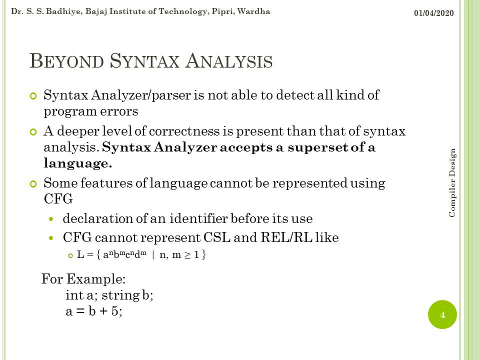 int a string. b. a equals to b plus 5.. You can see that this use of b on the right hand side of the expression is invalid, as we cannot add an integer value to this string and again assign it to a int variable. So this error is ignored by. 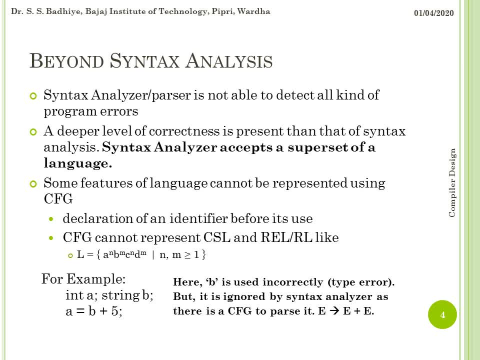 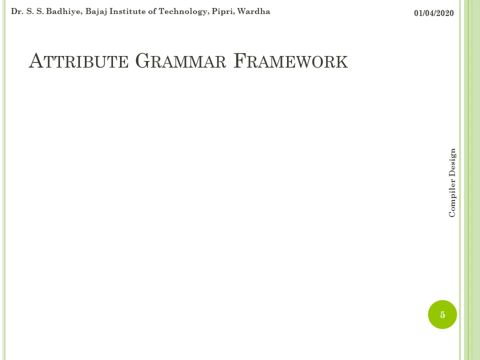 the syntax analyzer. as syntax analyzer can easily parse this input string by using a context free grammar of the type e derives to e plus e, which is also an expression grammar. We have already seen that an attribute is a property attached to each grammar symbol of the parse tree node. 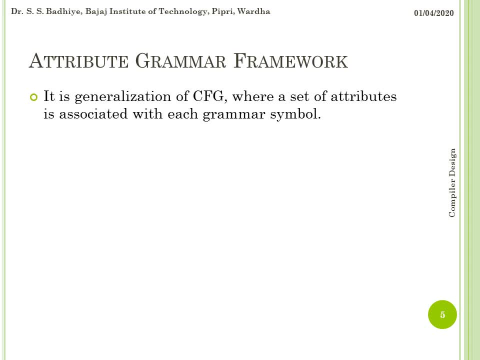 Attribute grammar framework is a generalization of context free grammar where a set of attributes is associated with each grammar symbol. The values of each attributes are computed by associating semantic rules with the production rules. Semantic rules are associated with the production rules in two different ways. 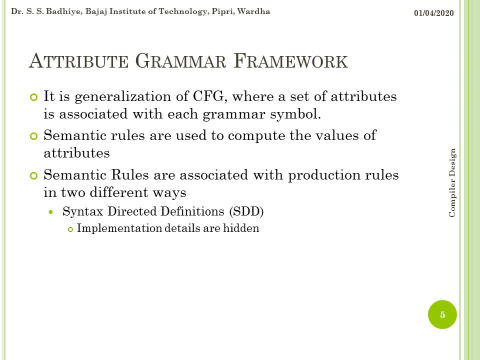 The first way is by using syntax directed definition. This syntax directed definition hide the implementation details from the user. It is high level specification of the context. free grammar. Order of evaluation of the parse tree is not specified in the syntax directed definition. Another way of associating semantic rules: 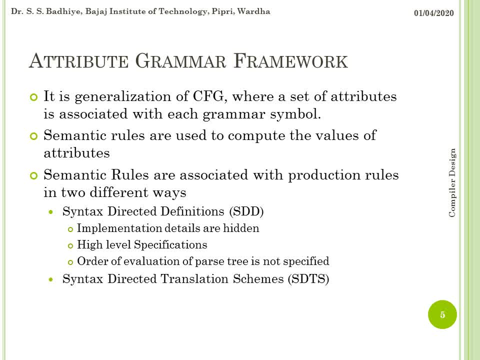 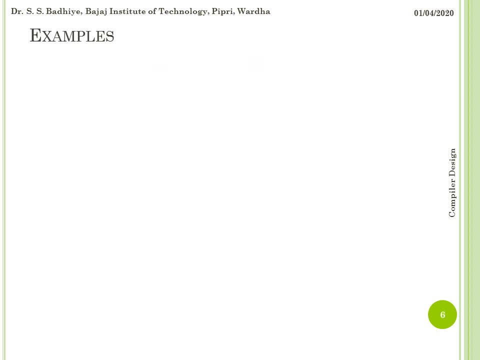 with the production rules are through syntax directed translation schemes. Here the order of evaluation is specified and some implementation details are also visible to the user. Consider the following example of declaring variables as: int. a, comma b, comma c. semicolon. The grammar or cfg used for this declaration is given. 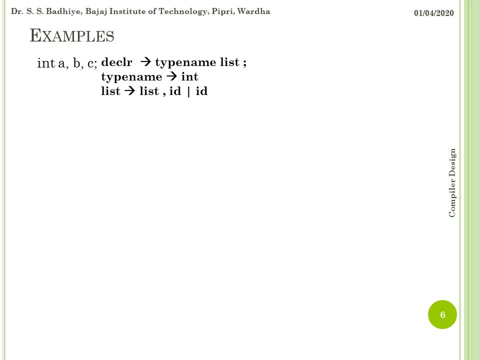 as: declaration derives to type name, followed by list semicolon. Type name derives to int, List derives to list comma id or list derives to id. The parse tree obtained after syntax analysis for the input int a, comma b, comma c semicolon is represented by the following parse tree: 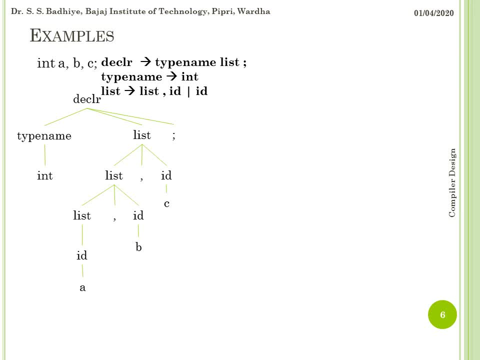 Here you can see that each node of the parse tree has some attributes associated with it. For example, type attribute is associated with each node- a, b, c, id, list, type name. The value of these attributes of any node is obtained from some other nodes in the parse tree, For example, 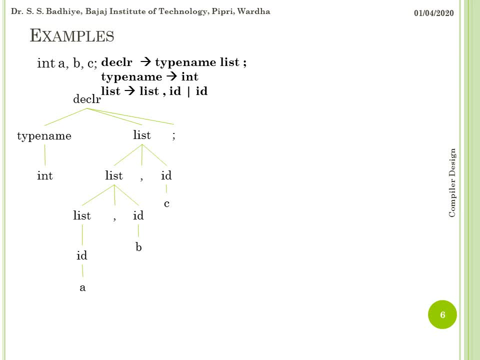 the first list here gets the value of its type from the type, name type- Whereas this value of the type of id is obtained from the first list which is above it, And the type of the second list is obtained from the first list, and so on. In this way, each 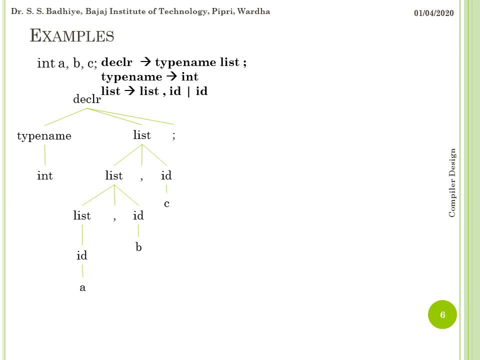 node of the parse tree is obtaining the value of its attributes through some other node, either across the tree or from any other way. Consider another example: Int a, string b, a equals to b plus c. The grammar used for this expression, a equals to b plus 5, is e derives. 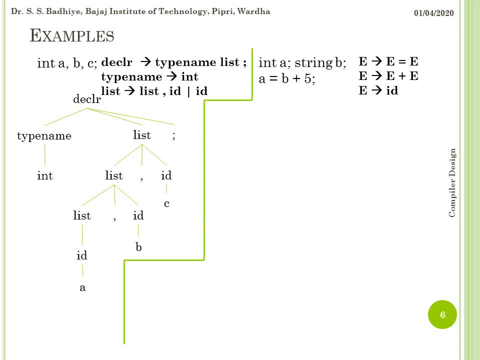 to e, equals to e, e derives to e plus e and e derives to id. The parse tree obtained after syntax analyzer for the expression is shown below. Here each node has some properties associated to it, like type, So the type of id is obtained from the lexical value. 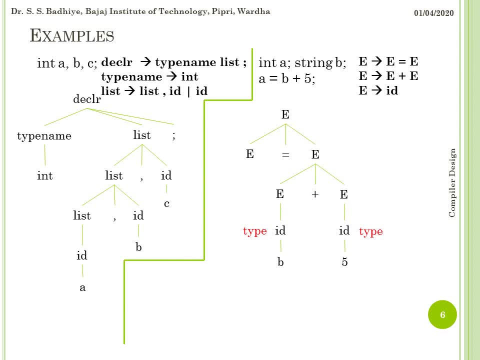 of that id which is stored by the lexical analyzer in the first phase, and this is obtained from the symbol table by using lex value or type lex type function. This type value is forwarded upward to the above node, that is, type of b. id is carried upward to the type of e, then type of. 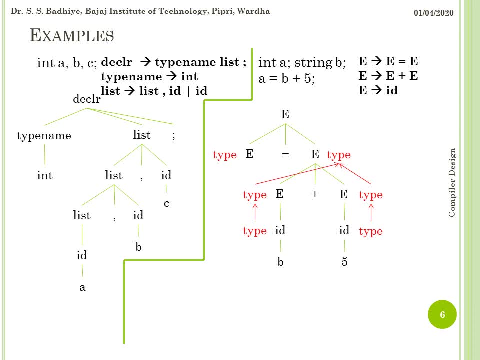 e is carried again upward to obtain the type of e, and then this type of two e's are again used to obtain the type of the topmost e. For this purpose, in case of syntax directed definition, we have to associate some semantic rules with each. 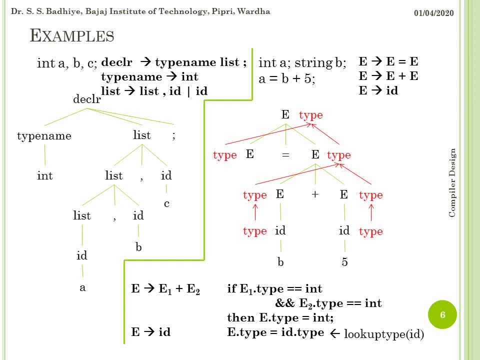 grammar production rule Here for obtaining the type of id. so we the type of id is obtained by using lookup type function which, through this symbol table which is associated with id dot type, then the value at this id dot type is given to e dot type. So whenever 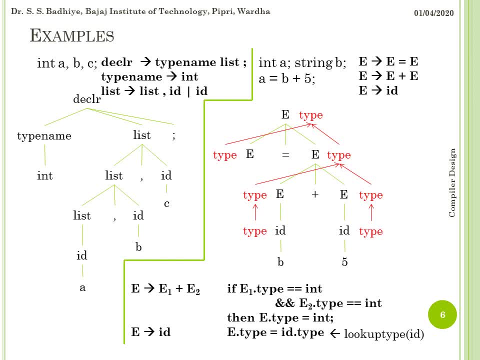 there is a reduction of the form, e derives to id, that is, whenever id is reduced to e. at that time e dot type will be assigned a value of id dot type. Consider another rule: e derives to e1 plus e2.. Here I am using the denotation. 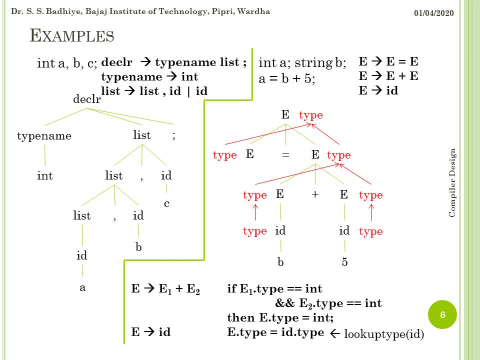 1 and 2, so as to separate all the occurrences of this e. Here the value of e dot type is obtained by using the value of e1 dot type and e2 dot type. So if e1 dot type is equals to, equals to int and e2 dot type is 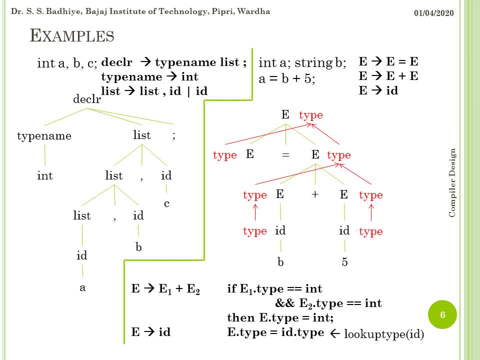 also equals to int, then e dot type will automatically become int. In this way we also write some other rules wherein if type of e1 and type of e2 is different, then it will perform some type correction, that is, forceful type conversion, or it should report certain errors. 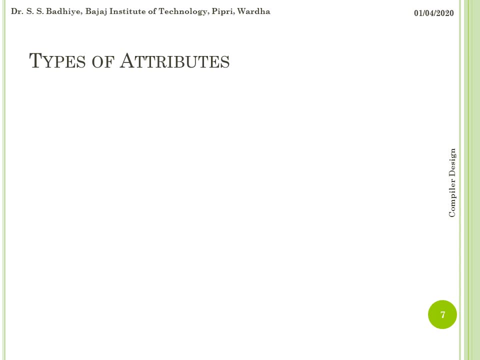 In the previous two examples, we have seen different ways in which values of attributes can be computed through semantic rules Based on the way an attribute is obtaining its value. there are different types of attributes. First are the synthesized attributes: If the value of any attributes depends upon the value, 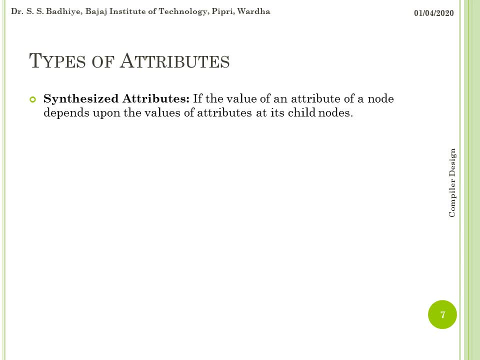 of attributes of its child node, then such type of attributes are called as synthesized attributes. Another kind of attributes are called inherited attributes. If value of any attribute of an attribute at any node is obtained from the value of its parent node or of its sibling node, then such kind of attributes are called as. 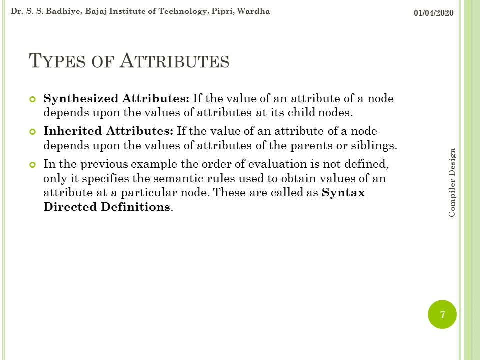 inherited attributes. In the previous example the order of evaluation is not defined, Only it specifies the semantic rules used to obtain values of the attribute at particular node. As the order is not specified, these are called as syntax directed definitions. If we need to associate 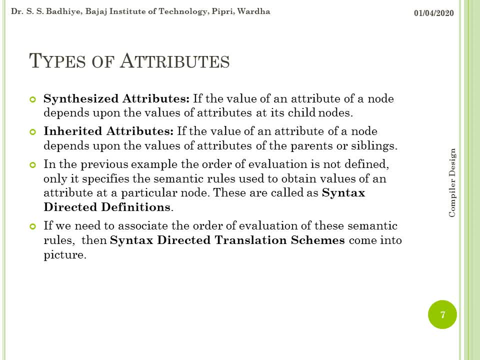 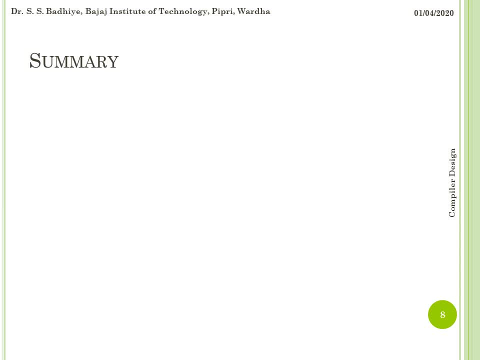 the order of evaluation to of these semantic rules. then syntax directed translation schemes come into the picture. Here we present the summary about SDD and SDTS. Conceptually, both of them parse input token stream. They also build parse tree. They traverse the parse tree to evaluate semantic rules at the parse tree. 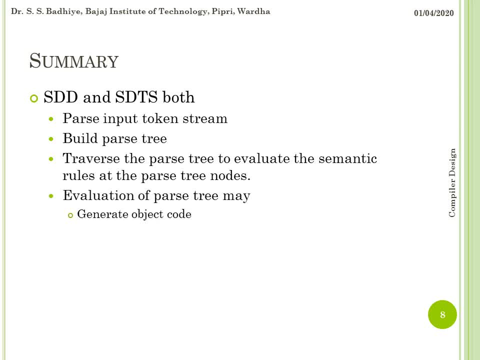 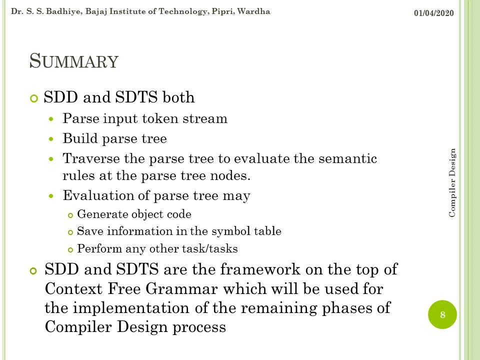 node. Evaluation of this parse tree may generate object code. It may also save information in the symbol table or it may perform any other task. SDD and SDTS are the frameworks on the top of the context tree grammar which will be used for implementation of the remaining phase of compiler design. 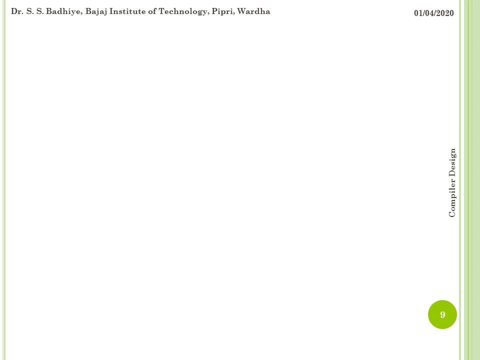 process. Here we are going to see how to write a syntax directed definition for a given grammar. Consider a grammar for signed binary number, which is given by the following rules: The next step is to build attribute grammar that annotates numbers with its value that it represents. So consider the following: 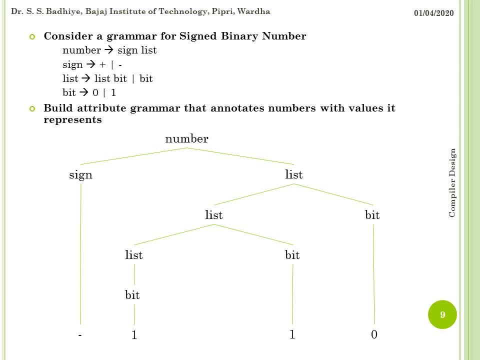 parse tree, which represents a number minus 6.. So the value of number is minus 6.. This is to be evaluated by using the syntax directed definition. For this purpose, we assign various properties to each node of the parse tree and we write certain semantic rules associated with each production rules. 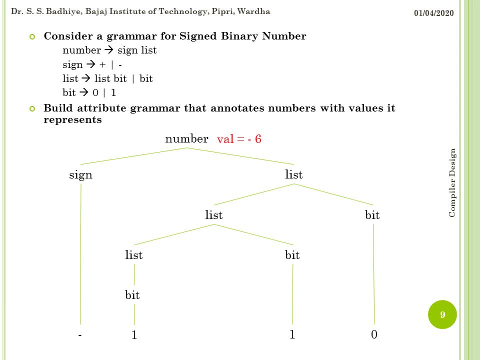 By using this semantic rules, we will be obtaining the values of attributes at each node of the parse tree. For the purpose of getting value as minus 6 at the root node, that is, val, equals to minus 6, we have to associate some attributes at each node. 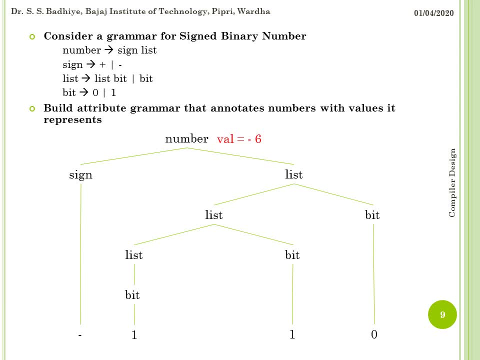 As we know that a binary number can be converted to decimal by considering the place value and multiplying with the face value and 2 to the power. what is the place value? So consider attribute position that represents the place value. So the place value of the first list that will generate the 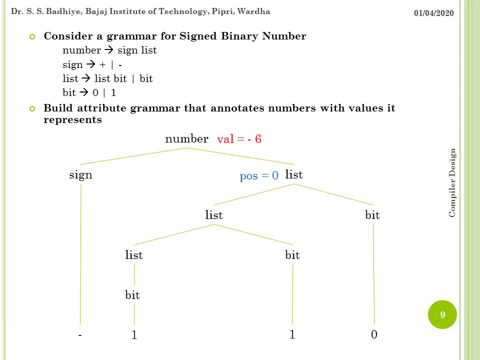 first bit will be 0. This position will be assigned to the bit which is generated by this list. Then the next list will generate another bit. So the position value of this list, or the new bit which is generated by this list, should be one more than this bit, the previous. 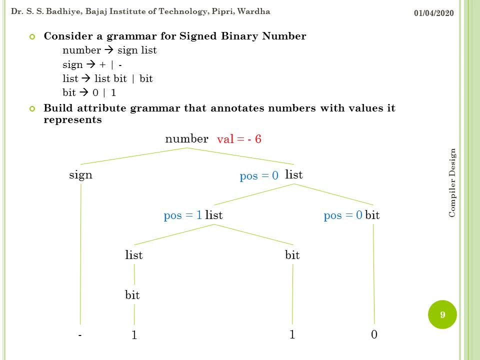 bit. So the value of position at this node shall be one more than the value of position at this first list node. So we increment the value of position at this list node and make it pos equals to 1.. Then the value of pos at the next level. 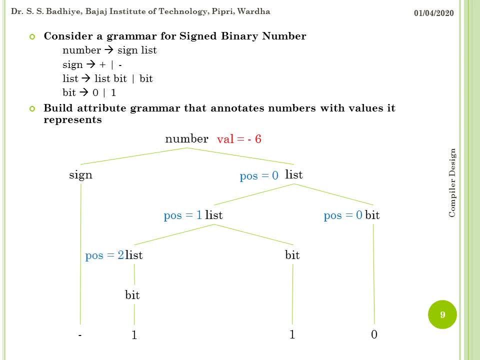 of list will again be incremented by 1.. So the value at the third list will become pos equals to 2.. Similarly, this value will be carried forwarded to the bit node and that will be equal to pos equals to 2.. Whereas the bit related to the first list will have the value. 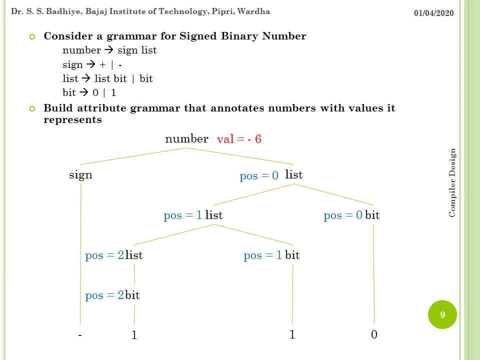 of position, which is equal to the value at the first list. So pos of bit will be 1.. Then the values of this is computed by considering the place value, that is position, and the face value, that is 1.. So the value at this bit is obtained. 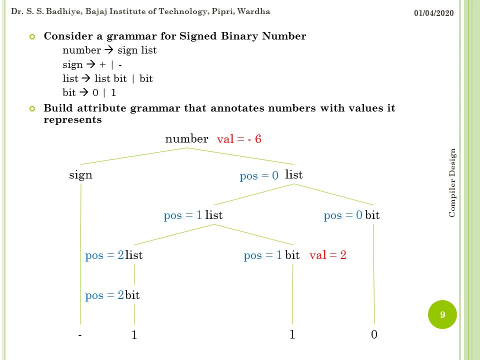 as value equals to face value into 2 to the power position, that is 1 into 2.. So the value becomes 2.. The value at this node, bit node, is obtained again by multiplying face value with the 2 to the power position, or the place value, that is 2 to the power 2.. So 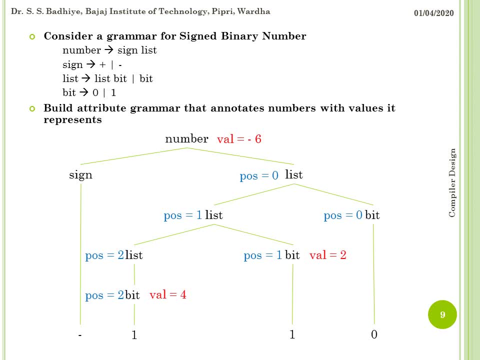 the value at this bit becomes 4, which is carried forwarded to the list. So value of list will be equals to value of bit. Here the value of list is obtained from its child node. So this kind of attributes are dash. They are called as. 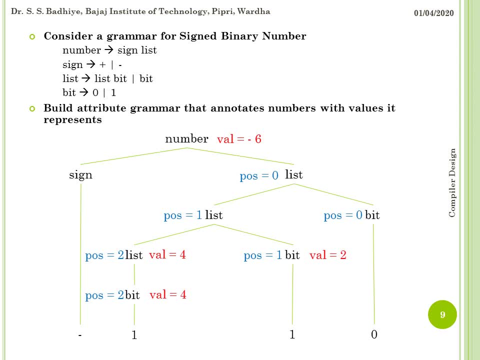 synthesized attribute. The value of this bit is again obtained by the same formula and it is found to be: val equals to 0.. Then the value at pos, list 1, is obtained from the value of list 2 and value of bit, That is addition of the 2. So the value becomes: 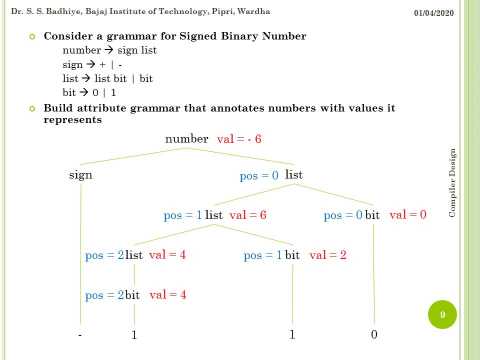 6. Unless all the nodes below this list is computed, we cannot compute the value of this list. So for computing value of this list, all the nodes below it shall be computed. To obtain value of first list we need value of first list and the value 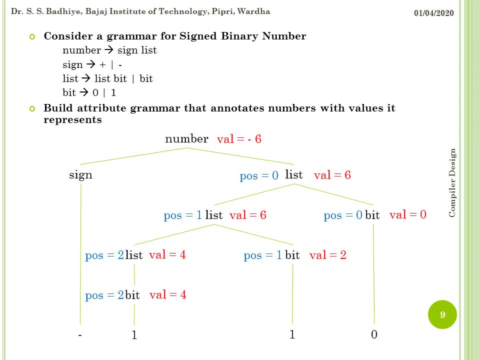 of first bit And we have obtained that. so the value of list will be equal to 6.. 0 plus 6, that is 6.. Similarly, the sign has an attribute associated with it- is pull, And the value of pull is false because it is negative. 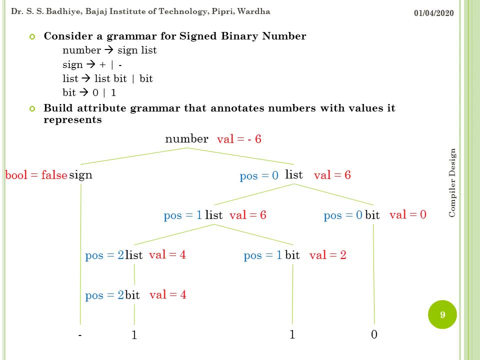 So when the value of this sign and list is obtained we can compute the value of number. So now val becomes sign. that is minus and val is 6. So this is minus 6.. Here some attributes like value. This is a synthesized attribute because the value of 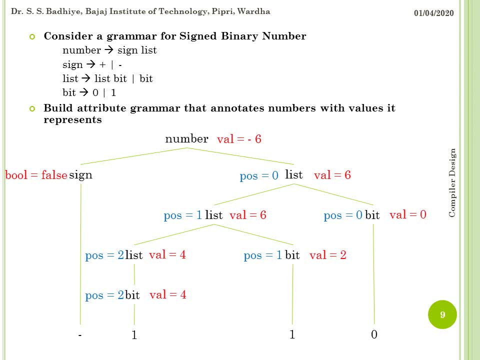 each attribute value at every node is obtained from its child node, Whereas the attribute position is of the type inherited attribute, as it obtained its value from the parent node or from the siblings. Here it obtained the value from the sibling- sorry- from the parent node. 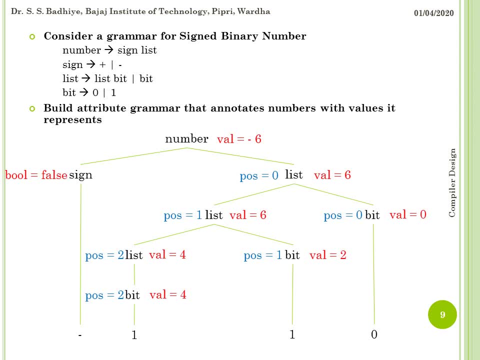 Here we have seen that the order of evaluation is not fixed. First we computed the value of list bit, then we computed the value of this list, then this list bit, and the order was not fixed, as the order of evaluation or obtaining value of the attributes was not fixed. 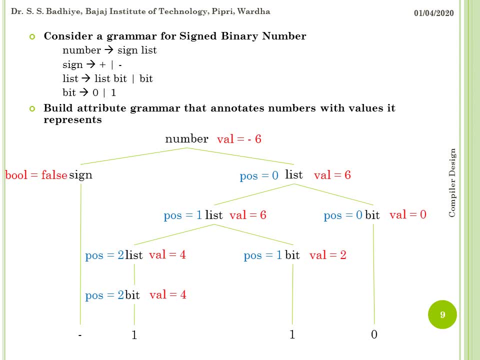 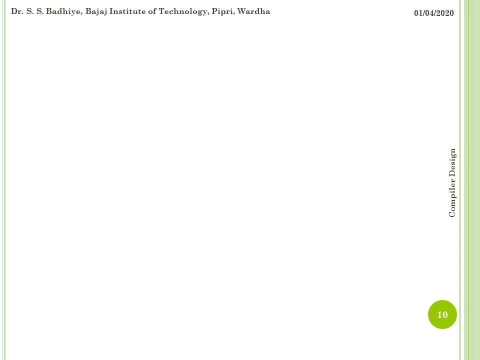 Therefore it is called as syntax directed definition. as the order is not fixed over here, This kind of pass tree having an additional properties at each node is called as decorated pass tree or annotated pass tree. In the previous slide we have computed values of attributes at each node Here. 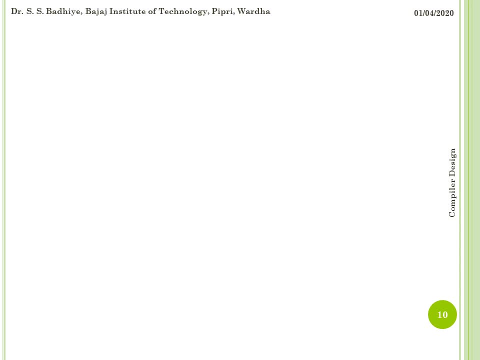 in this we will be writing the rules that we used for each production for obtaining the values of its attribute. Consider: the first production number derives to sign, followed by list. The semantic rule associated with it will be the value of attribute. position for the list will be given as for the first list will be assigned as 0. 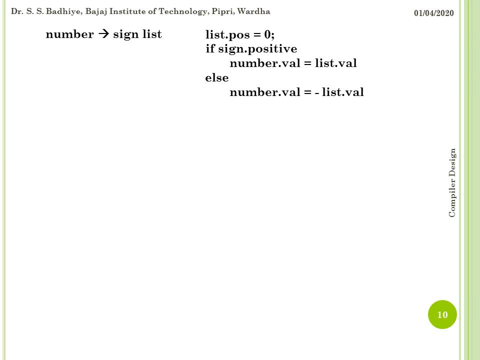 that is, list dot position, will be equals to 0. and if the value of bool attribute is sign dot positive? if it is positive, then the value of the number node, that is, number dot value, will be equals to the value that is present at the list, that is, list dot value. or if 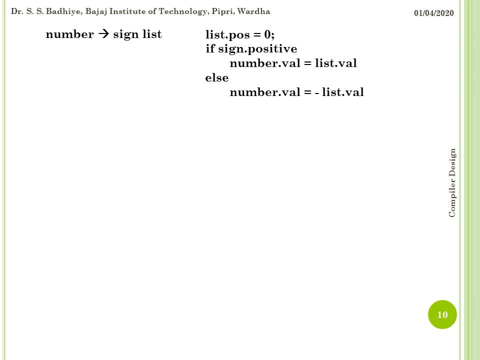 sign is negative, then the value of the number, that is, number dot value attribute, will have the value as minus of the value which is present at the list node, that is list dot value. Consider another rule: sign derives to plus and sign derives to minus, So the semantic rules associated. 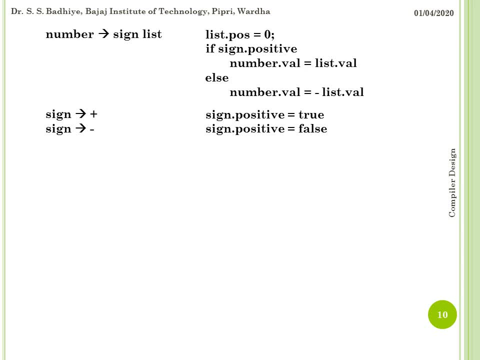 to. it is: sign dot positive is equals to true if sign derives to plus and sign dot positive is equals to false if it is negative. These are bool values. Consider the next rule: list derives to list1 dot, followed by bit. This one is just to separate. 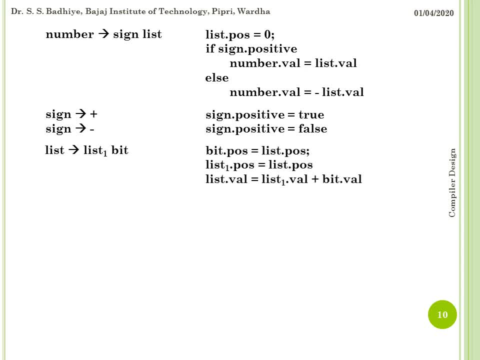 the occurrence of first list and the second list. The rules associated to this production are: the value of the position attribute for the bit node is obtained from the left hand side. that is the parent node list. that is list dot position. so bit dot position is equals to list dot position. 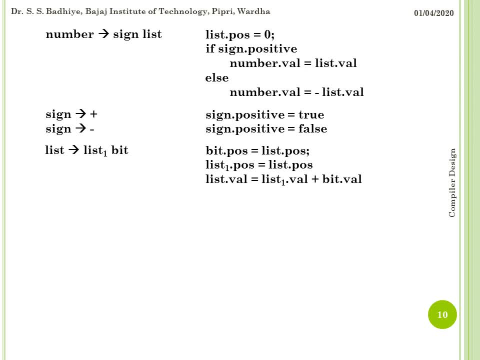 the value of position at list1 is obtained from the value of the list position, so value of list1 position is equals to the value of the list position, whereas the value at the list node is obtained as sum of the value of list1 node and the value of the bit node. So list1- list dot value. 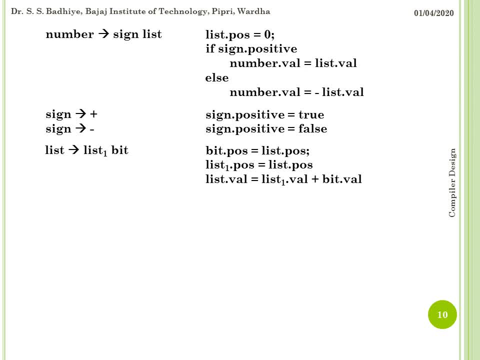 is equals to list1 dot value plus bit dot value. Consider the next rule where list derives to bit. Here the position value of bit is the position value of the list and the value of the list is equals to value of the bit, that is, list dot val is equals to. 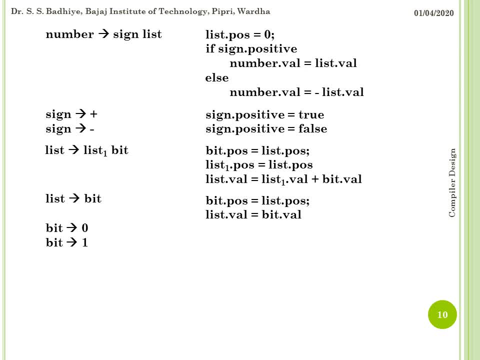 bit dot val. If bit derives to 0 and bit derives to 1.. If bit derives to 0, then the value at the bit node that is bit dot val is 0, and if bit derives to 1, then the value at the bit node that is bit dot value. 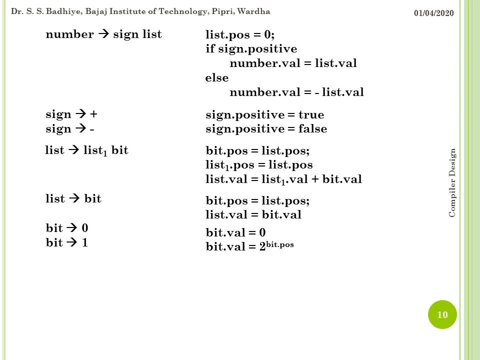 is equals to 2 to the power bit dot position. whatever is the value of the position of bit. The next step is to associate attributes with the grammar symbol. So for writing SDD we need to associate. these are just an example of rules that we will be writing. 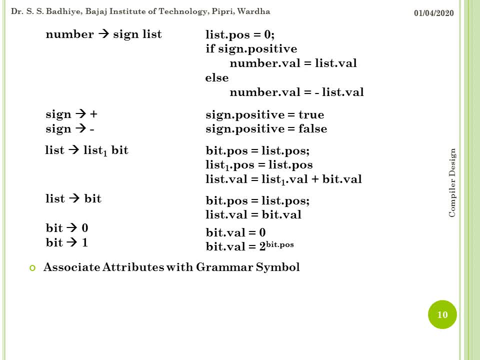 Now the next step: after deciding these rules, we have to associate what are the attributes that would be required for writing SDD, related to every grammar symbol. So for number, we will have only one attribute, that is, value attribute. For sign, we will have boolean attribute, bool attribute. For list, we will have position. 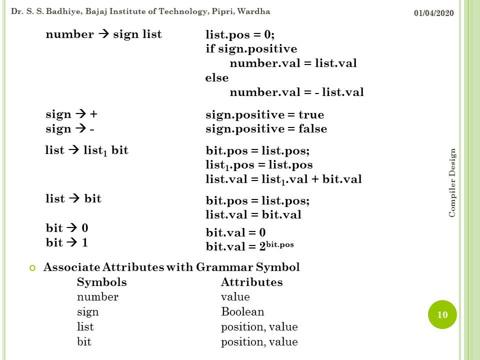 and value For bit we will have position and value as attribute. In the above example there is an error. that is list dot. list derives to list 1, followed by bit should have list dot position. that is list 1 dot position should be equals to list dot. 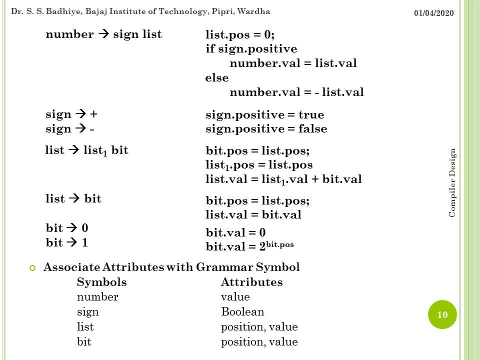 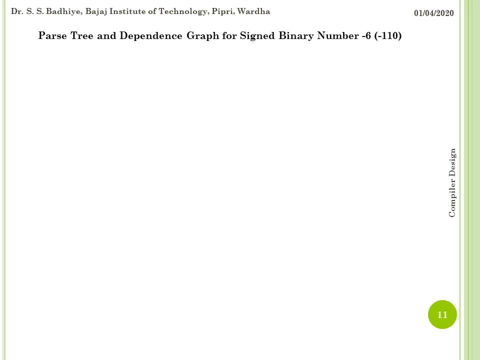 position plus 1.. Here there should be plus 1.. Once the syntax directed definition has been written, then we can find the values of any attributes at any node by traversing the parse tree, and at each reduction we will be executing the semantic action which is written. 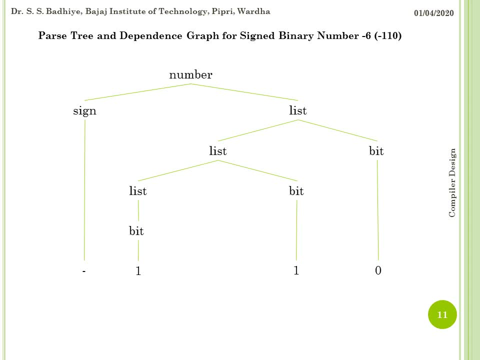 in front of that particular rule Here- consider the previous example- We can also draw the dependence graph from that particular derivation. So here from the rule we have obtained that position for the first list, node is 0.. The value at the second list and the bit is: 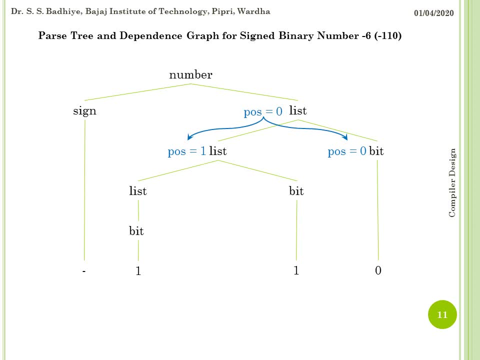 obtained from the position value of the first list. The value at the bit node is equal to the value of position at the list node, Whereas the value at the second list is equal to the value of position at the first list plus 1.. Then this value at list 1 is: 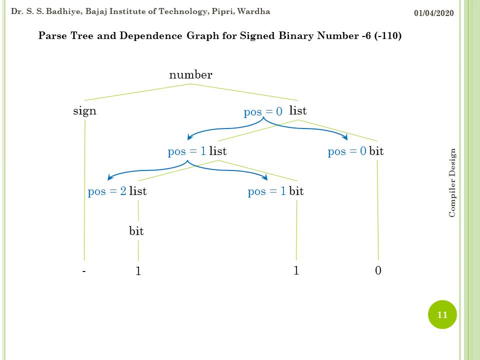 again carried forward to the next level and the value of this list of position is given as the same value to the bit node. So at bit node the value of position will be 1. Whereas this position value is incremented by 1 to get the value of the third list, that is, position will be. 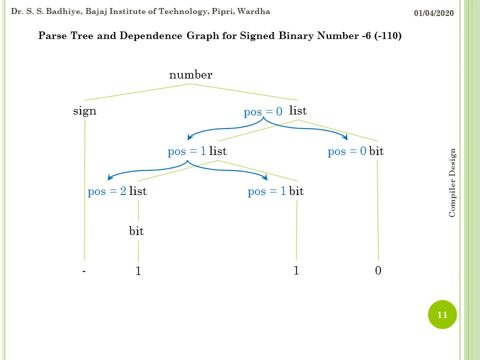 incremented again by 1.. So pos of the third list will be 2.. Then this position value is again carried forward to the next level of the node bit and the value at this list position is equal to the value at the bit position. In this way the values of attributes are carried. 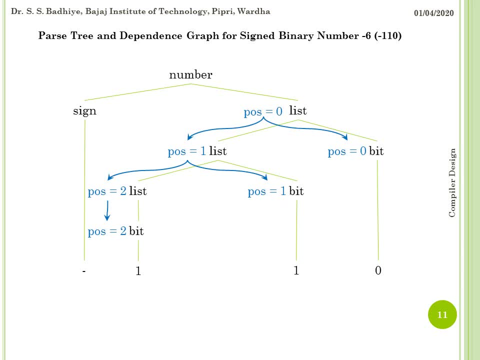 forward from the parent node to the child node. Every time this position attribute is forwarding the value from the parent node to the child node, Such attributes are called as synthesized or inherited Think. they are called as inherited attributes because the nodes at the lower level are obtaining the value. 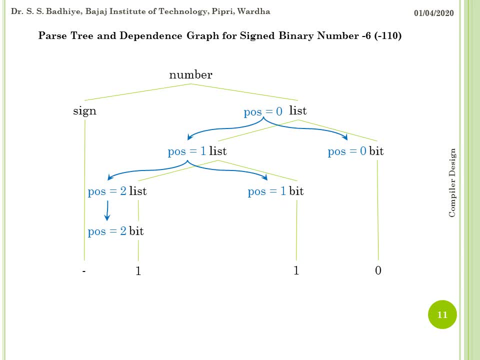 from their parents or from siblings. So this kind of attributes are called as inherited attributes, Whereas when the value of any node is obtained from its child node, then such attributes are called as synthesized attributes. So here the next attribute is value. So the value of first bit is obtained. 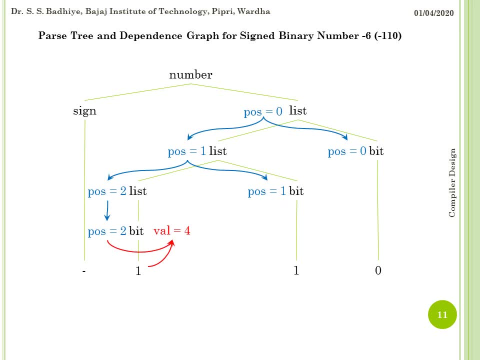 by considering the position attribute, the value of the position attribute and the face value, So it is computed to be 4.. Whereas this value is again forwarded to the, is carried upward to the list node and the value at this list node is equal to 4, which is equal to the value at the. 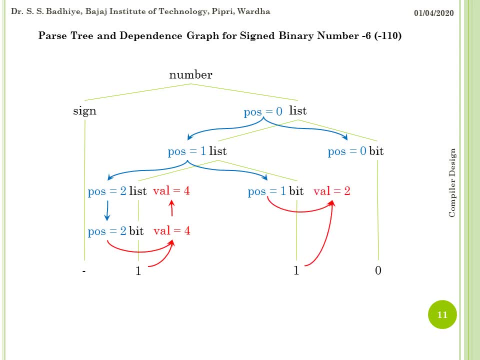 bit node. Then the value of second bit is obtained by the position value at bit node and the face value, So it is getting the value 2.. When we have obtained the value of list and bit, we can compute the value of the second list. So it becomes: 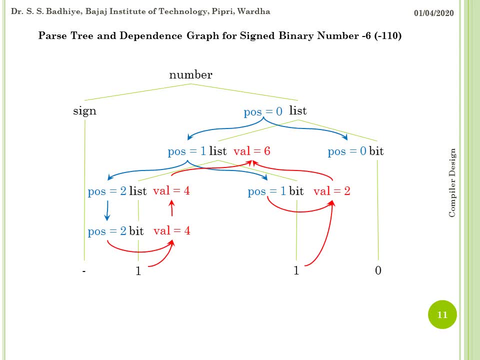 it is obtained from the child nodes, so it becomes 6.. Again we can compute value at the bit node- first bit node, as value equals to 0. Because the face value is 0 and position value is also 0. Once we have computed the value at this level for list and bit, 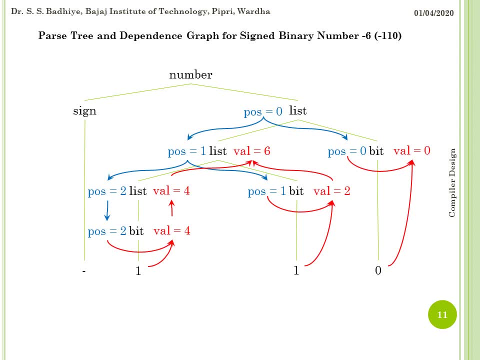 we can compute the value of the value attribute at the first list, which is addition of value at list 1, and value at bit, which is equals to 6.. The value of sign is false. Then again, the value of number is obtained from the sign node. build pull. 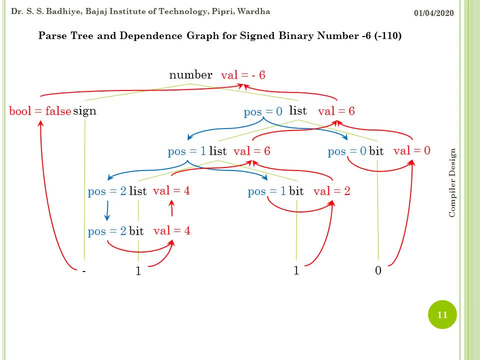 and the list node. So the value at number is minus 6.. Here we can see that the value of the attribute well is always carried upward from the child node to the parent node. So such kind of attributes, wherein node obtain values from its child node, are 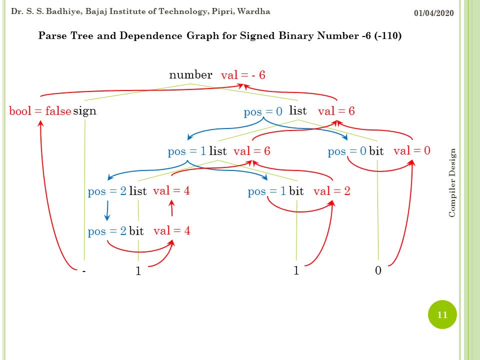 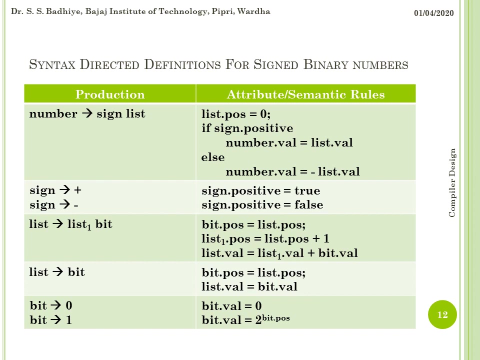 called as synthesized attributes. So here we have seen both kind of attributes, that is, inherited attribute and synthesized attribute. Position pos is inherited attribute, whereas val is a synthesized attribute. So this slide shows the production along with the semantic rules. So this is syntax directed definition for signed binary numbers. 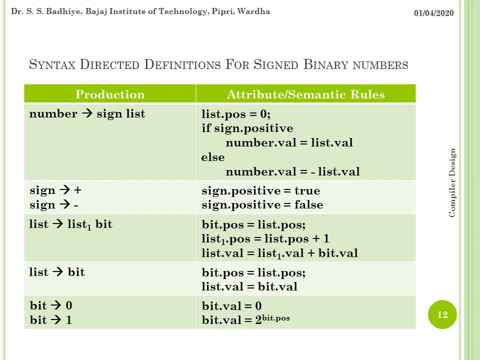 Here there was a mistake in the previous slide, that is, list 1 dot position was equals to list dot pos. Here you need to write plus 1.. So this is the correct way of writing. syntax directed definition. Here the order of evaluation of this semantic rules is not fixed. You can evaluate bit. 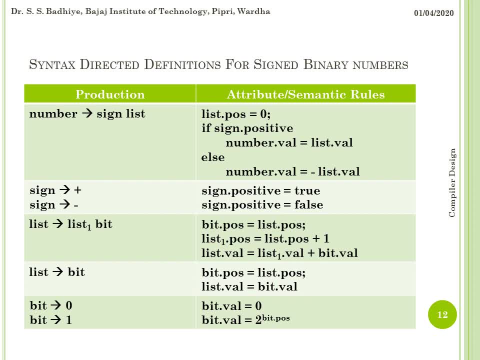 derives to 0 first, bit derives to 1 later, or bit derives to 1 first and then bit derives to 0, and any occurrence of list 1 or list you can evaluate in any order. So the order is not specified over here. So these: 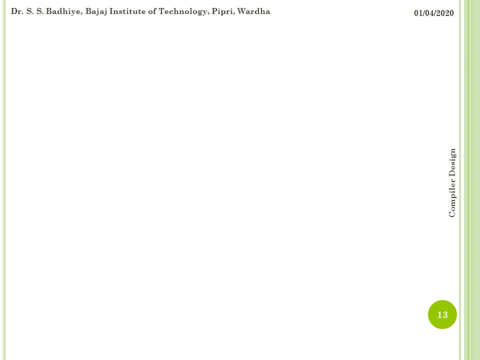 are called as syntax directed definitions. Let us consider another example for writing syntax directed definition for a calculator program. The grammar is given below. We need to build an attribute grammar that annotates number with the values it represent. Consider the following parse tree Here: the: 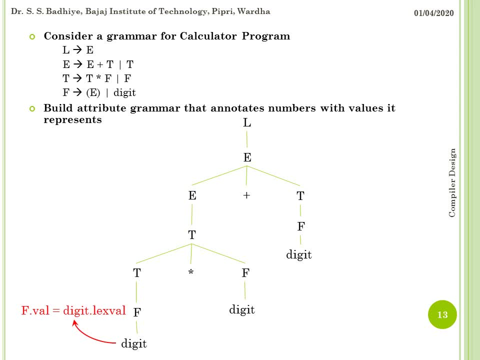 each node is have assigned an attribute val. So the value at the f node for the attribute val is obtained by the lex value of the digit. This lexical value of digit is stored by the lexical analyzer into the symbol table. So this can be obtained by: 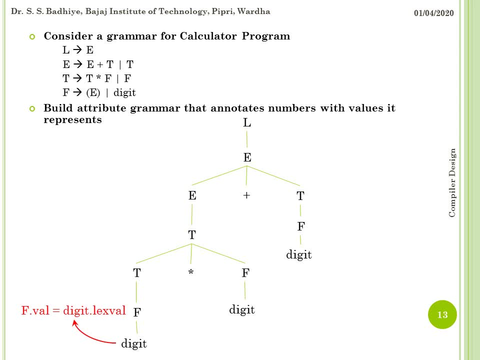 the function lexval. So the value of digit dot lexval is assigned to f dot val, which is carried upward to the t nodes and the value attribute at the t node is computed as t dot val equals to f dot val. whenever there is a reduction of the form, t derives to f. 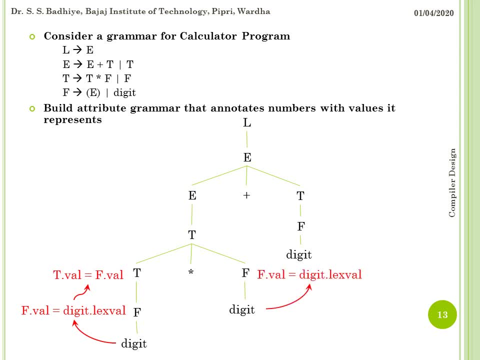 The value of the second f f dot val is again obtained by digit dot lexval. These two values of t and f are carried forward to the upper t and the value at this t node is obtained as t dot val equals to t one dot val plus. 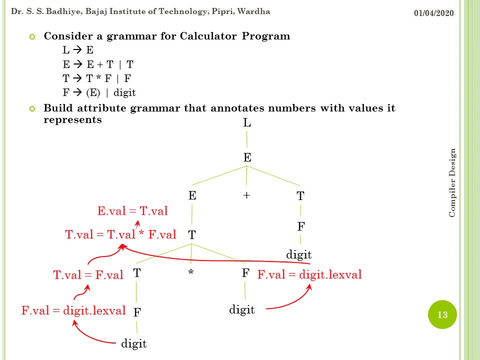 f dot val. Once this is computed, it is carried forward to the upper node, that is e, and the value at the e node is e dot val equals to t dot val. The f val at the first f is obtained by digit dot lexval, which is carried upward to the t node. 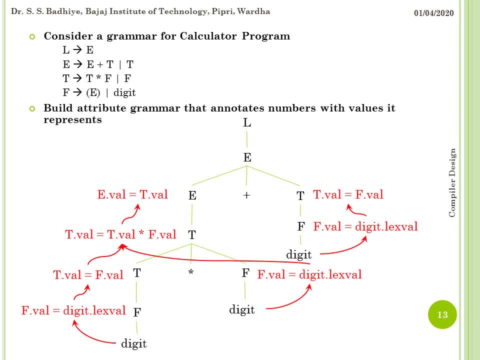 to give t dot val equals to f dot val. These two values at the e plus t e node and t node are carried forward to the e node to obtain e dot val equals to e dot val plus t dot val and the value at the first node, that is l. 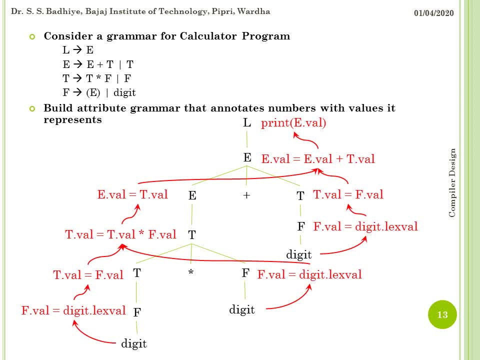 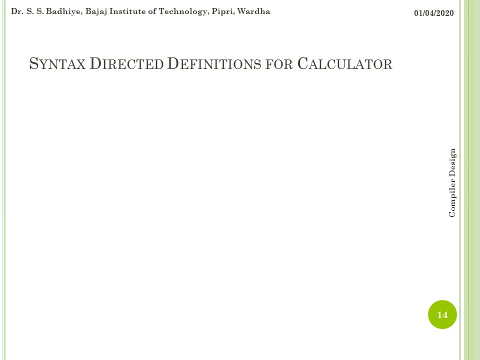 is performed by the action of printing the value at e dot val. Whatever is, the value at e dot val will be printed by the calculator. whenever there is a final reduction from e to l, The syntax directed definition for the calculator is obtained from the previous as. 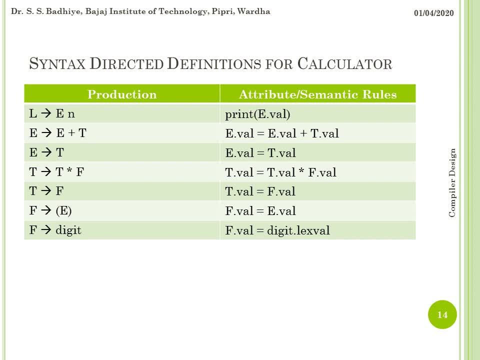 follows. So the rules associated with each production rule are written over here. that we have already discussed in the previous slide. You can go through the rules. All the terminals here are assumed to have only synthesized attributes, So the value of all terminals are: 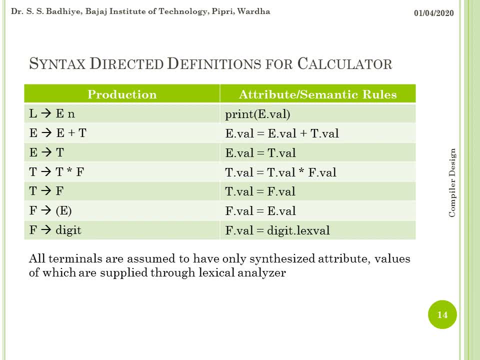 supplied through the lexical analyzer. Hope you remember that lexval function. A syntax directed definition that uses only synthesized attributes is said to be s attributed definition. Based on the types of attributes that a syntax directed definition uses, it is divided into two types: s attributed definition and l. 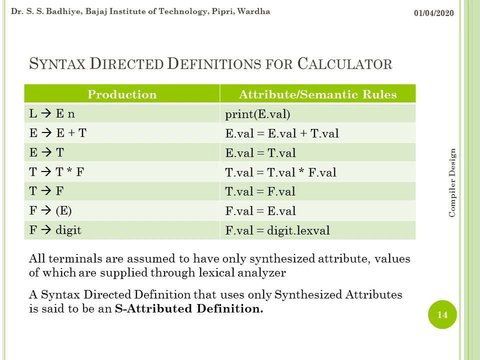 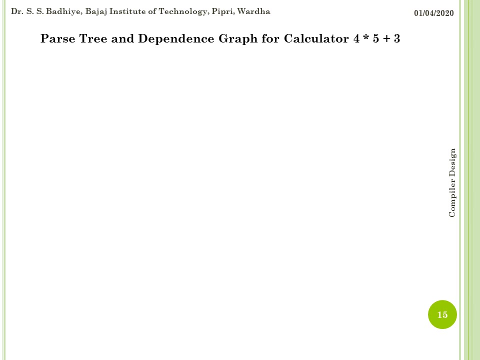 attributed definition. If a syntax directed definition consists of only synthesized attributes, then it is called as s attributed definition, whereas an l attributed definition can have both inherited as well as synthesized attributes. By using the syntax directed definition defined in the previous slide, we have to obtain a parse tree and dependence graph. 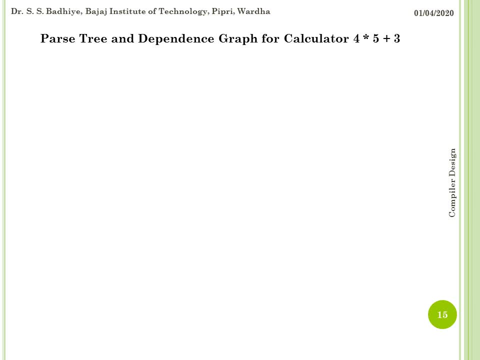 for calculating the following expression: 4 into 5 plus 3.. A parse tree of an s attributed definition can be annotated by evaluating semantic rules of the attributes. So this is the parse tree which is obtained from syntax analyzer for the given expression, and the value at the f node, as we have seen, is computed. 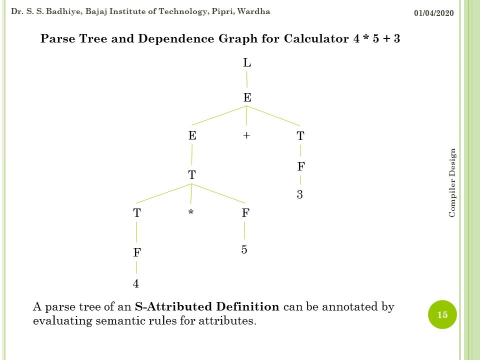 as the lexval of id. Here lexval is the face value, that is, 4.. So fval gets value 4.. This value, 4, is carried upward to the value of t node, that is, tval equals to 4.. The value: 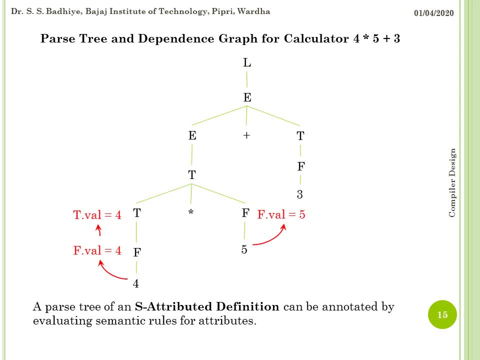 at this f node is fval equals to the lexval of this id, which is 5.. This is carried forward upward to the t nodes and it is obtained as 4 into 5.. So the tval at this node is equals to 20, which is again carried. 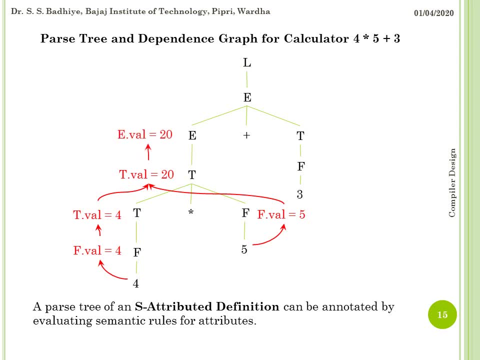 forward to e node, that is eval equals to 20.. Then the value at this f node is the lexical value at this node, which is 3.. So fval is 3, which is carried upward to tval equals to 3 and the eval is obtained as: 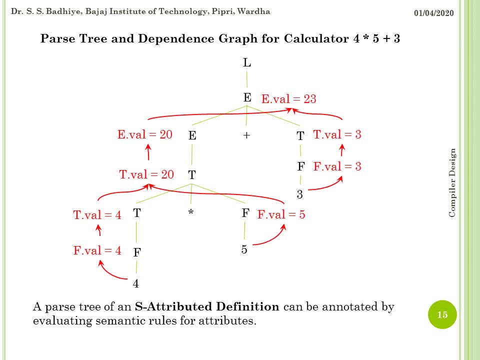 e1.val plus tval, which is 20 plus 3, that is 23, and when the final reduction is there- e derives to l- will print the value 23 on the output screen. So this graph wherein the arcs show the dependency of obtaining value, 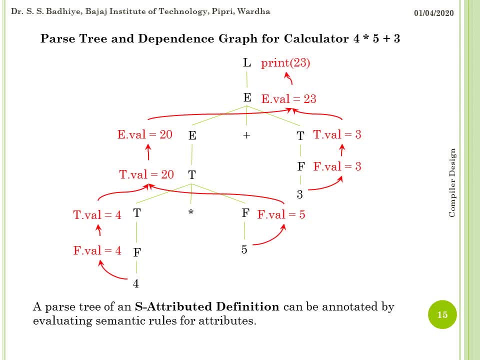 of each attribute at the nodes, like the value of f, cannot be obtained if we have the lexical value of id. the value of tval cannot be obtained until fval is computed, and so on. So this shows the dependency of an attribute at a particular. 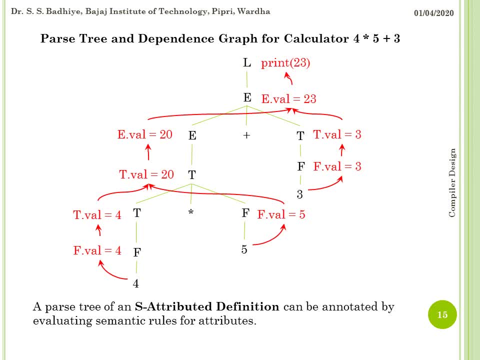 node. Thank you, Thank you.